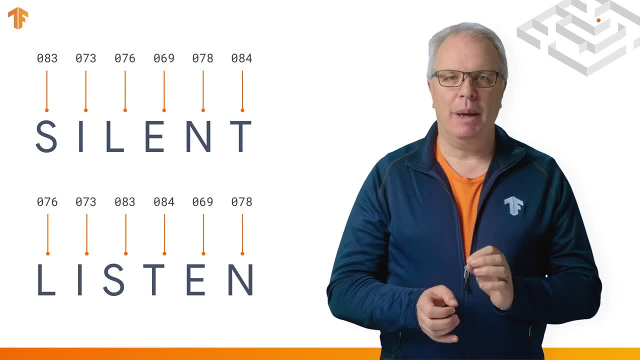 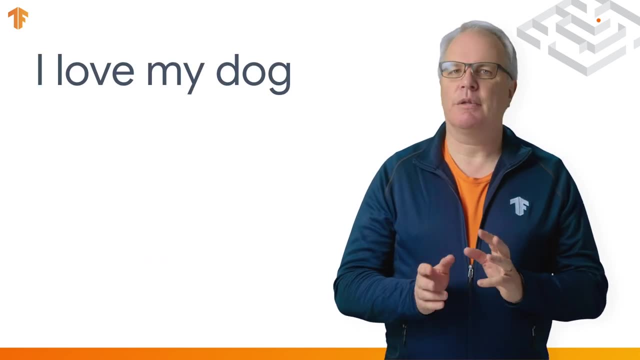 and thus the same numbers just in a different order. So it makes it hard for us to understand sentiment of a word Just by the letters in it. So it might be easier, instead of encoding letters, to encode words. Consider the sentence: I love my dog. 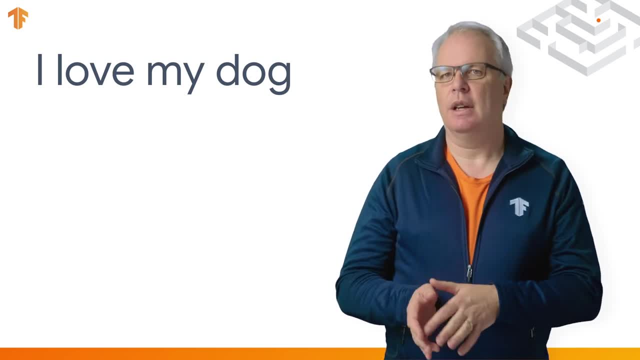 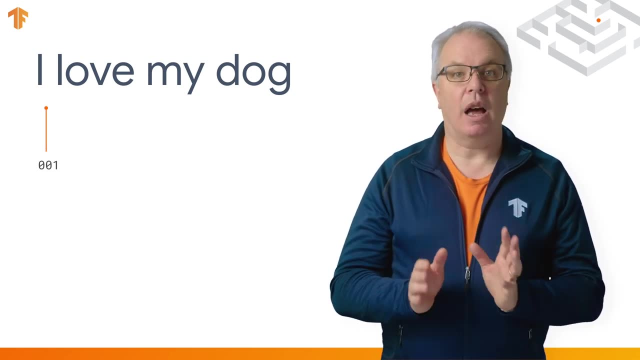 So what would happen if we start encoding the words in this sentence instead of the letters in each words? So, for example, the word I could be 1.. And then the sentence I love my dog could be 1,, 2,, 3,, 4.. 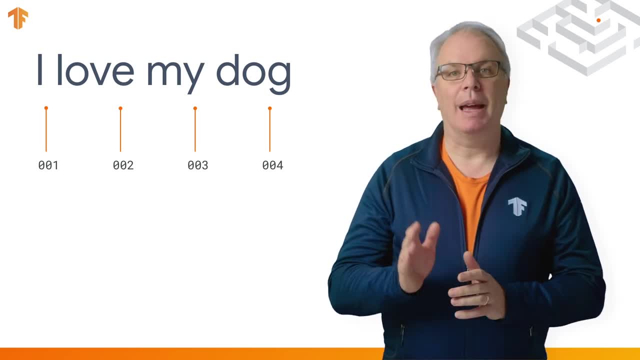 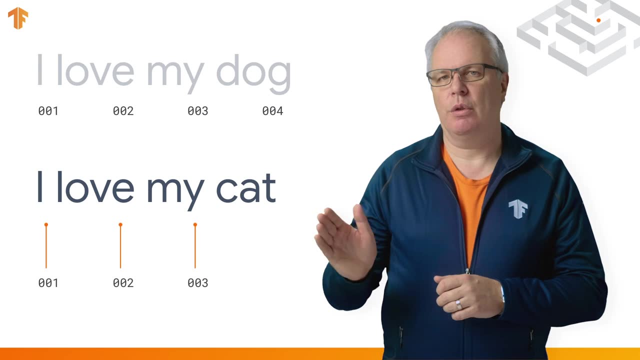 Now, if I take another sentence, for example, I love my cat, how would we encode it? Now we see, I love my has already been given 1,, 2,, 3.. So all I need to do is encode cat. 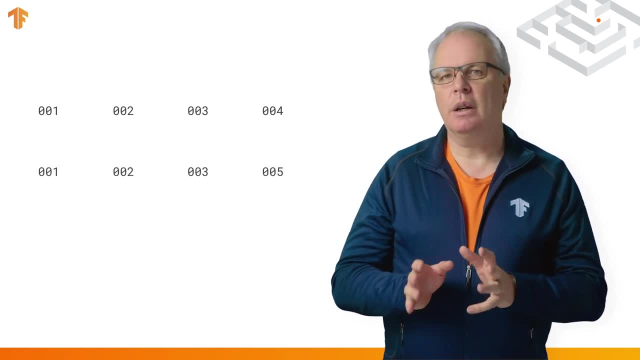 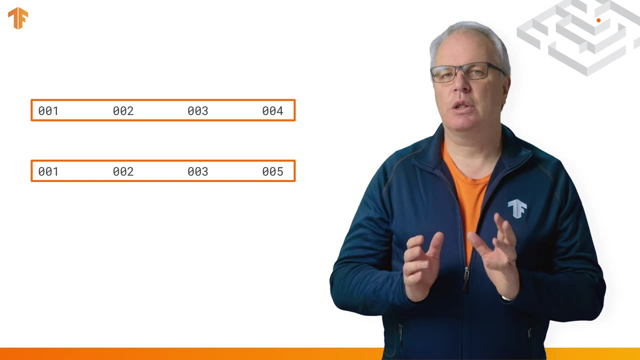 I'll give that the number 5.. And now, if we look at the two sentences, they are 1, 2, 3, 4, and 1, 2,, 3, 5,, which already shows some form of similarity between them. 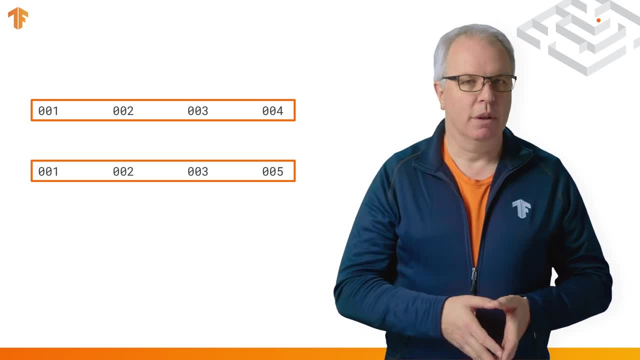 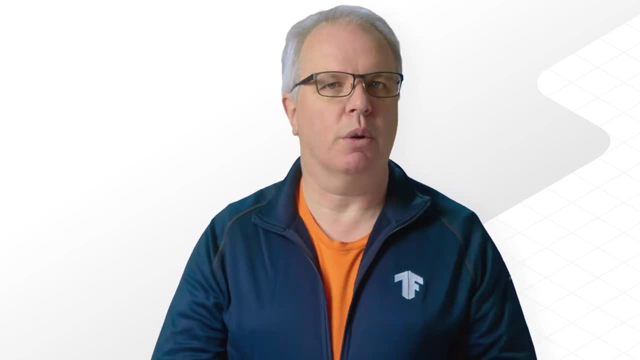 And it's a similarity you would expect, because they're both about loving a pet. Given this method of encoding sentences into numbers, now let's take a look at some code to achieve this. for us, This process, as I mentioned before, is called tokenization. 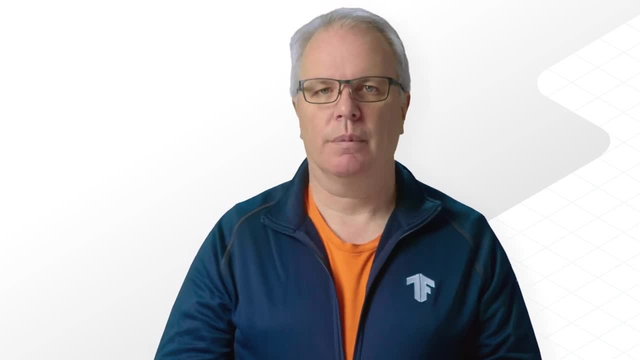 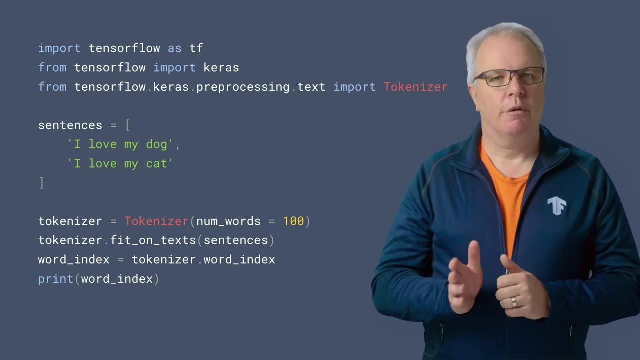 And there's an API for that. We'll look at how to use it with Python. So here's your first look at some code to tokenize these sentences. Let's go through it line by line. First of all, we'll need the tokenizer APIs. 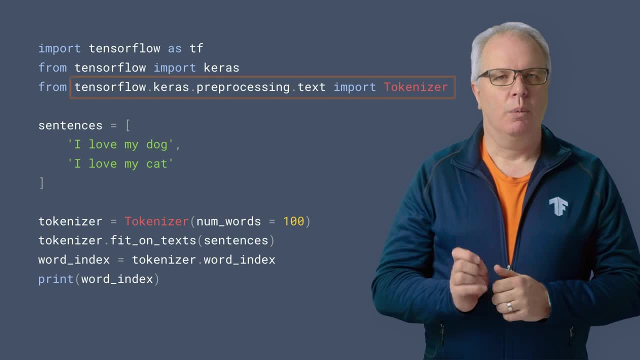 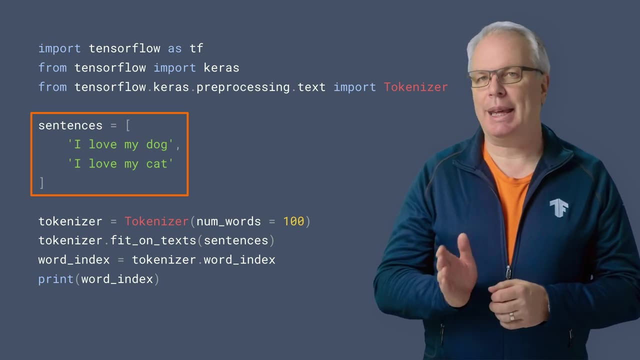 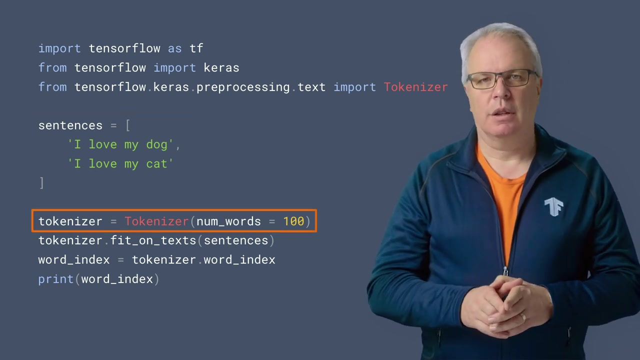 And we can get these from TensorFlow Keras like this: We can represent our sentences as a Python array of strings like this: It's simply the I love my dog and I love my cat that we saw earlier. Now the fun begins. I can create an instance of a tokenizer object. 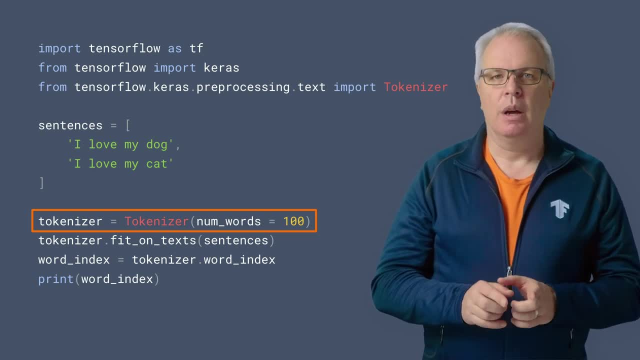 The numWords parameter is the maximum number of words to keep. So instead of, for example, just these two sentences, imagine if we had hundreds of books to tokenize, But we just want the most frequent 100 words in all of that. This would automatically do that for us.